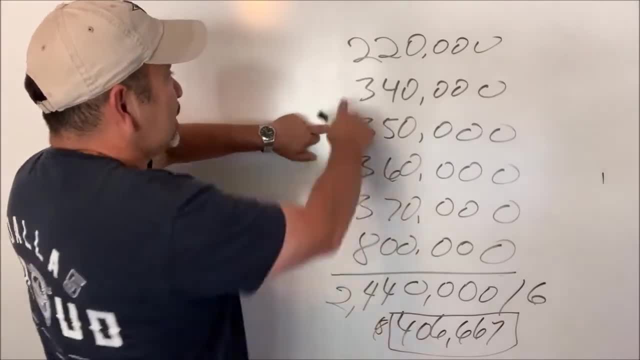 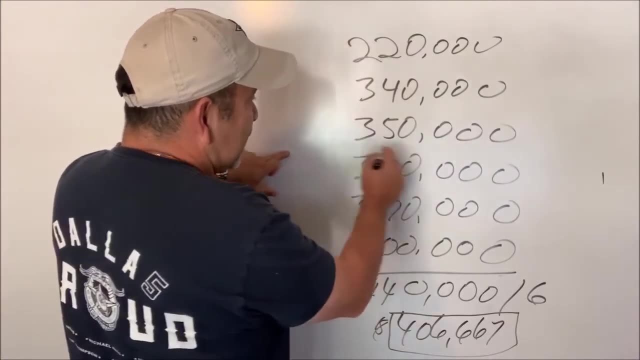 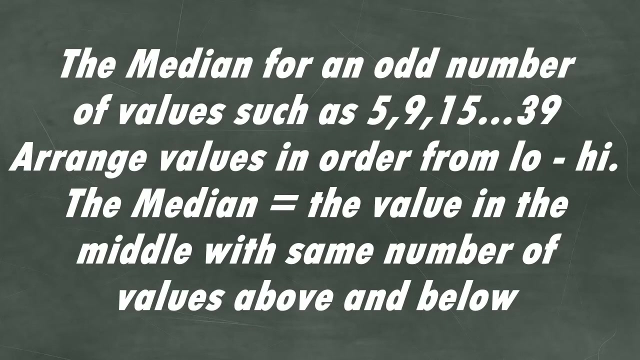 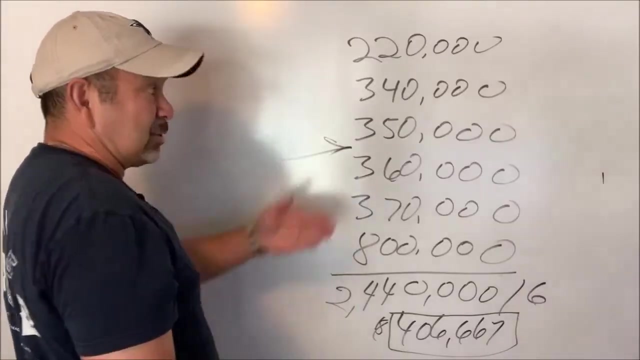 and three numbers there. So that can't be the middle Same with this one, Two numbers here, three numbers there, That kind of. We'd have to have an odd number of values here. So whatever number would fall right in here would actually be the median. But since we don't have one to get the median for two. 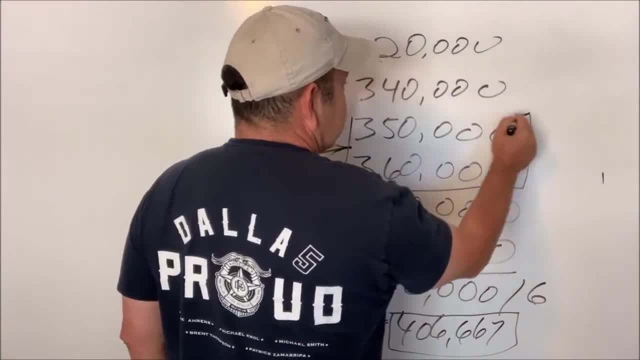 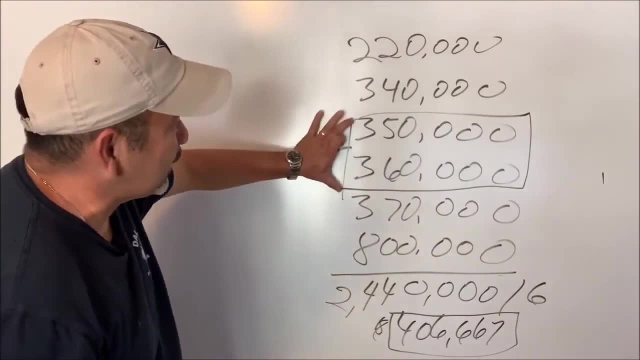 of them. If you have an even number of numbers here- This is six- You take these two, add them up and then divide them by. So you take the average of just the two values, which right here is going to be 710, divided by. 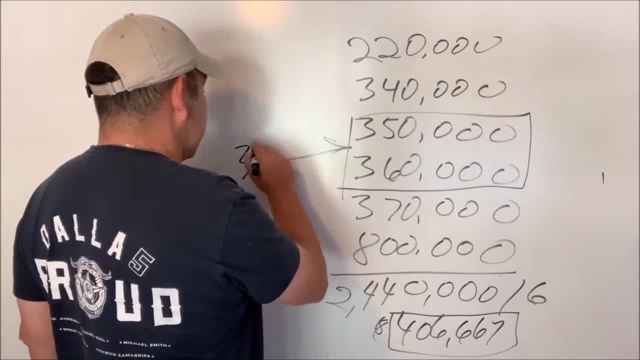 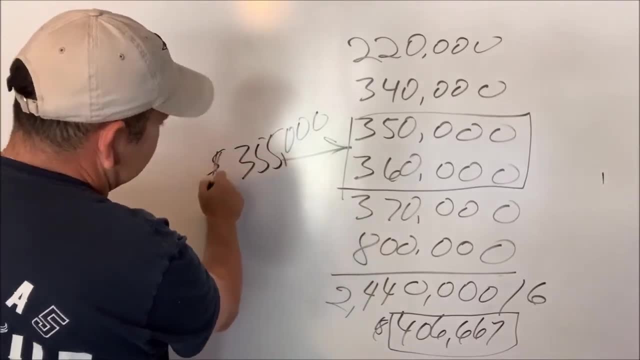 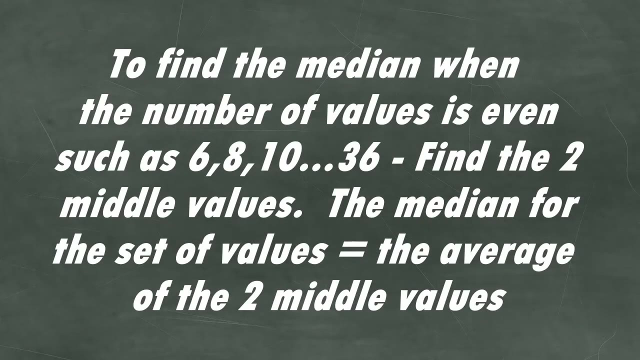 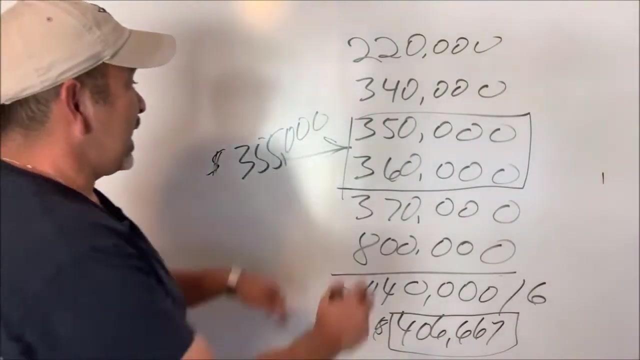 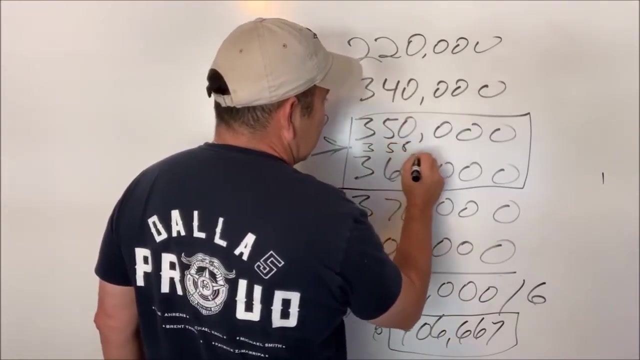 2 be 355.. So your median would be 355.. That's a big difference between this number and that number there. Now, if you had a number here that was, say, 358.. Say this: Say you had seven numbers here. And if you had here 358.. Believe it or not, the median would be this number here, 358.. 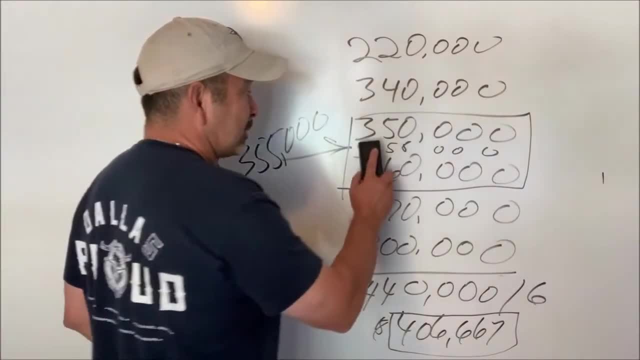 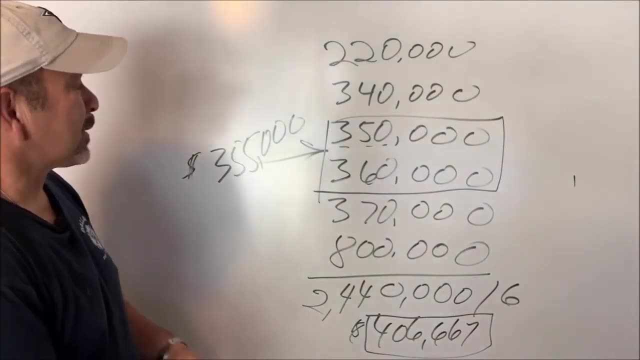 That's, if you had the seven numbers instead of six And this number, we got six numbers, So we're going to stick with that for now. So you're probably wondering: why do they use a median and an average? Well, if you look at this average, it's 406.. It falls above all of these that are in the middle. 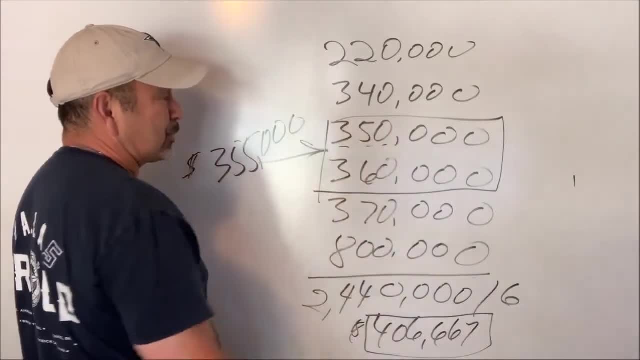 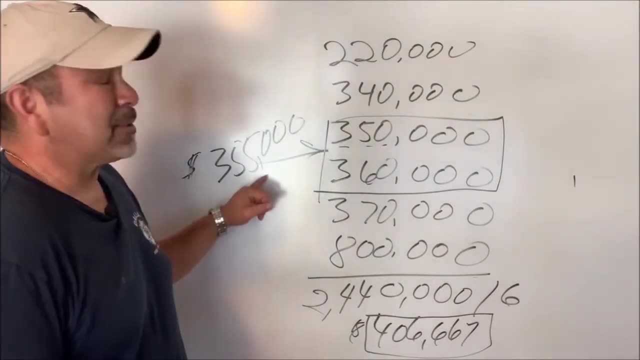 So the average or the median would give us a closer range or closer value of what is truly expected in that area. Now, another reason is the median. Most calendar reports zip codes or cities. They pull in all the data So they can't throw any of. 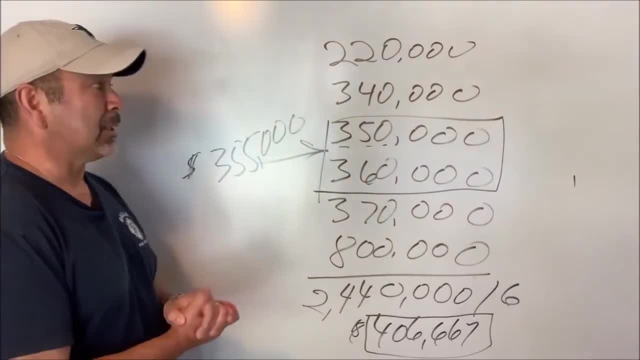 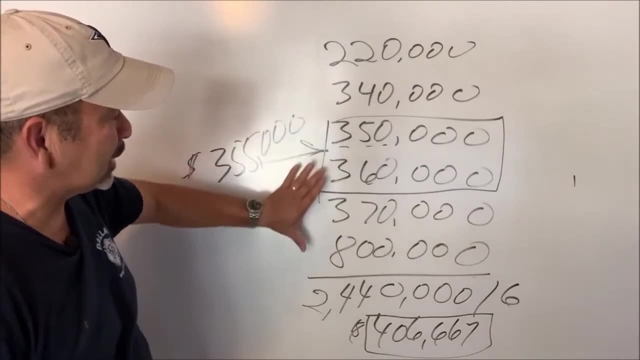 the numbers out. So they can't throw any of the numbers out. So they can't throw any of the numbers out. When an agent is analyzing your property, more than likely they're going to be looking at the area and the comps that are most likely close to your property. It could be these three. It could. 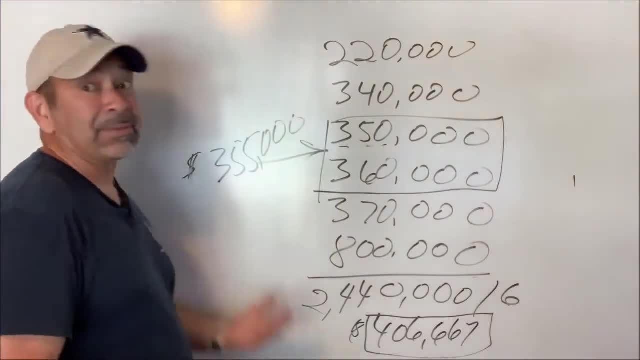 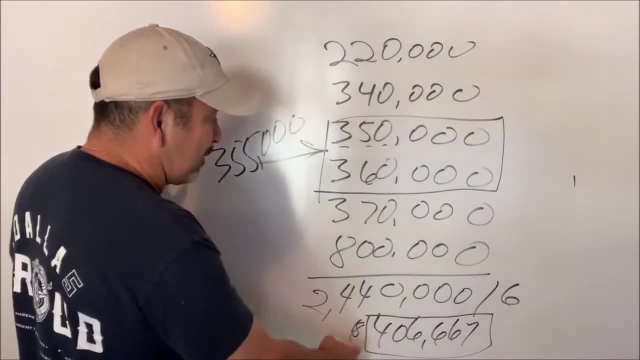 be these three And they're going to give a compare. you know, apples with apples. They're going to try to narrow in and give you a value on your house. Now listen, just because this is the median, that's the average, doesn't mean you can't get this If these houses here